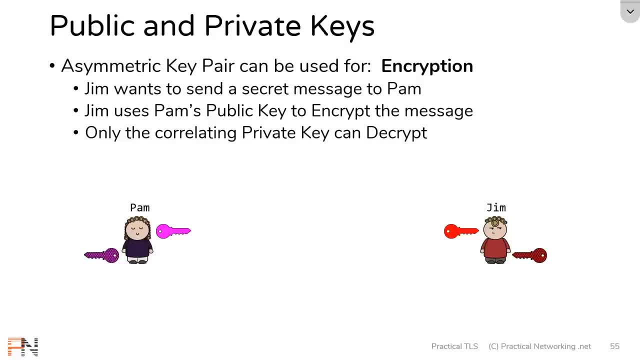 and extract the original plaintext, And this is how asymmetric keys are used to provide confidentiality. Recall that confidentiality is the idea that the data is only accessible to the intended recipient, And we can use an asymmetric key pair to ensure data confidentiality. But that's not all you can do with a set of asymmetric keys. There's actually something. 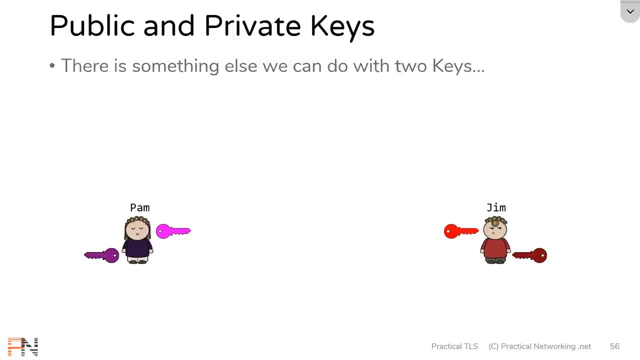 else you can do, which is pretty cool. Let's say, PAM now has a message for Jim. Let's say, for this particular message, PAM doesn't care about the confidentiality, meaning she doesn't care who can read this message, But she definitely wants to prove. 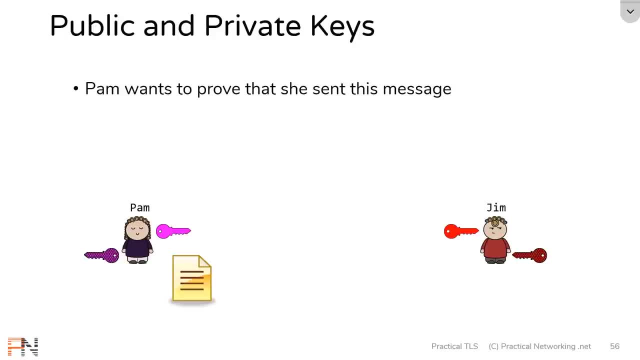 that it was definitely her that sent this message. What she can do is use her own private key to encrypt that message, And she can also use her own private key to encrypt that message. Now, the only key in the world that can decrypt that would be her public key. 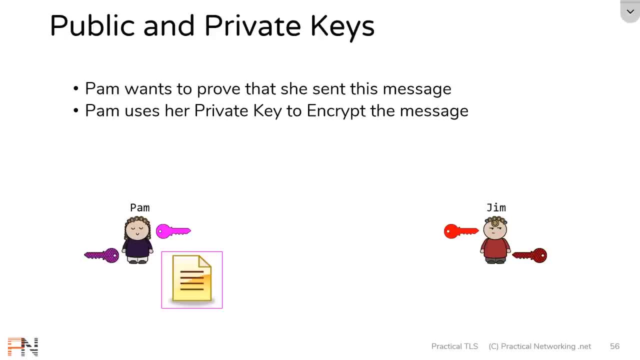 which Jim has and anybody else has, because it's a public key. So this can get sent across the wire And then Jim can decrypt that message using PAM's public key. If Jim can decrypt the message successfully with PAM's public key, this actually proves two things. First, it proves that PAM 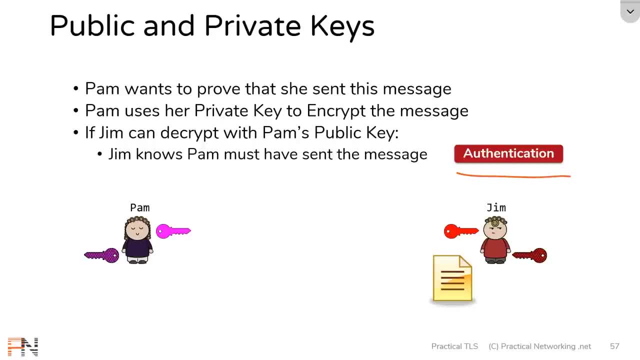 must have sent that message. This gives us authentication. If Jim was able to decrypt something with public key, it proves that the only key that could have encrypted it was PAM's private key, And PAM should be the only person that has that key. 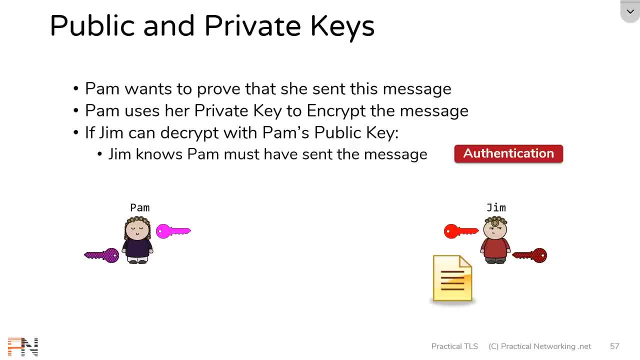 Therefore, we know PAM sent that message. It also proves something else. It also proves that the message was not modified in transit. That is integrity. If someone captured the message in the middle and changed the content of the message, well, when Jim tried to decrypt it with PAM's 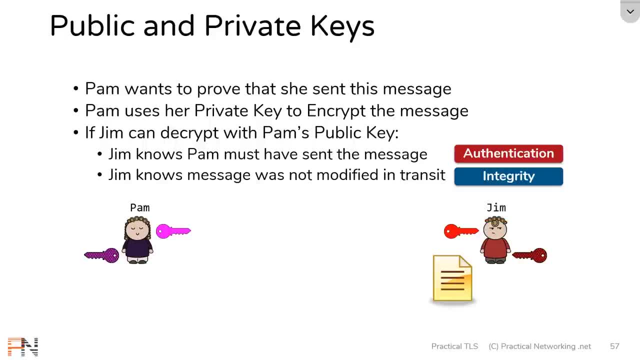 public key. he would end up with a message that was not encrypted. So this can get sent across the wire. So this can get sent across the wire. So this can get sent across the wire. So this can get sent up with a jarbled mess, if the decryption would have worked at all. So if Jim was successfully. 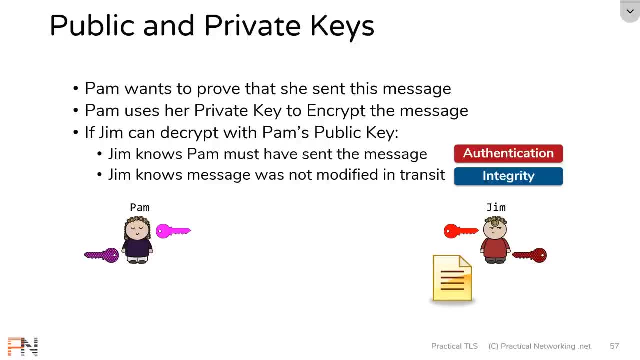 able to decrypt a message with PAM's public key, then we know for a fact the message hasn't changed since PAM encrypted it with her private key. This process that we just discussed is what's known as message signatures. You can use an asymmetric key pair to create a signature. 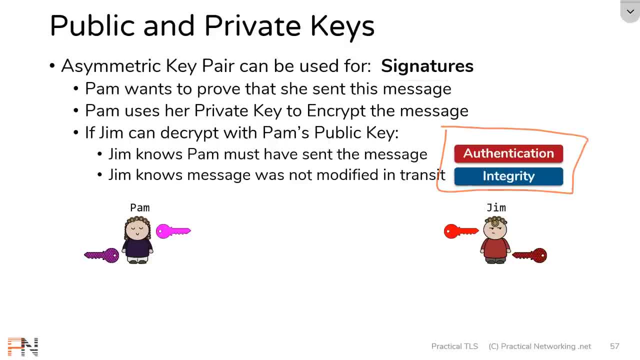 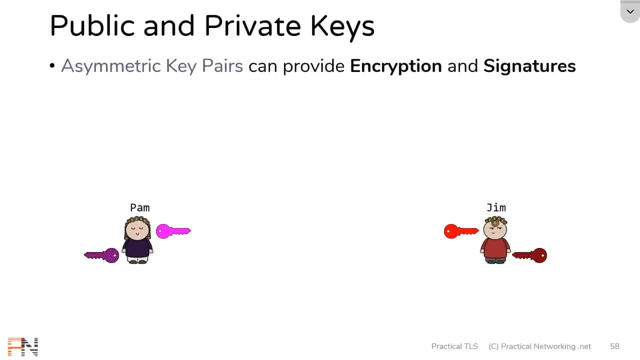 which provides authentication and integrity for what was signed. So we just talked through how you can use an asymmetric key pair to provide both encryption to get confidentiality, and signatures to get integrity and authentication. But in reality it's not quite that simple. Remember, in the last lesson we talked through 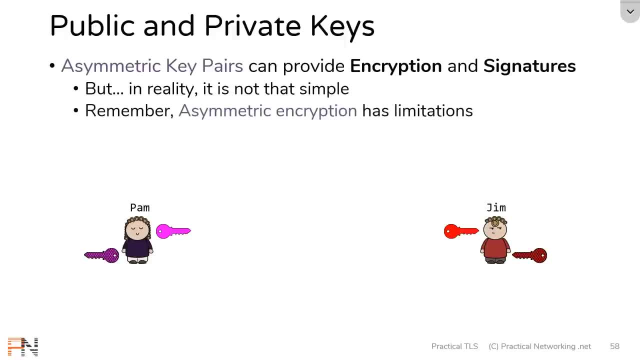 a bunch of limitations that asymmetric encryption has, namely, that it's inefficient to use asymmetric encryption for bulk data transfers, because asymmetric encryption is slower and more taxing on the CPU. Instead, if we want to actually protect bulk data, what we want to be doing is using symmetric. 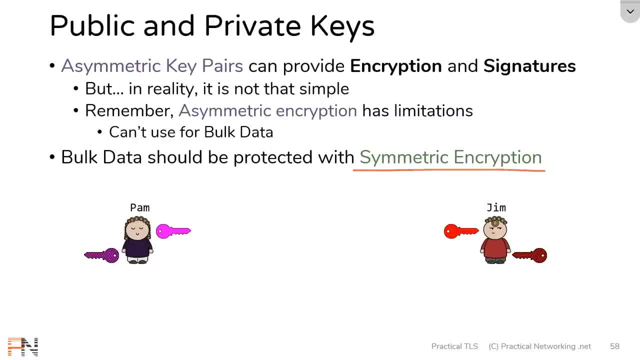 encryption, But symmetric encryption has this problem that we have to first establish a symmetric key on either side of the wire and we have to do it in a secure way. Well, that symmetric key is a pretty small piece of data And recall that we can use asymmetric 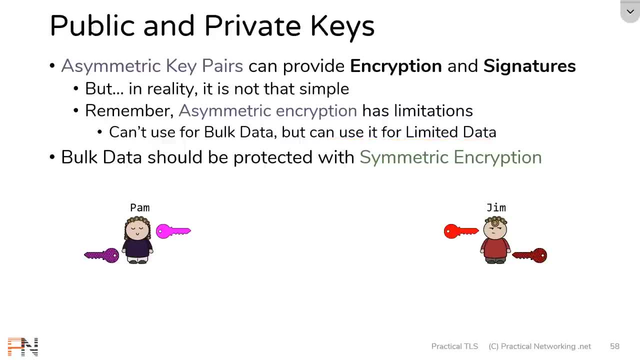 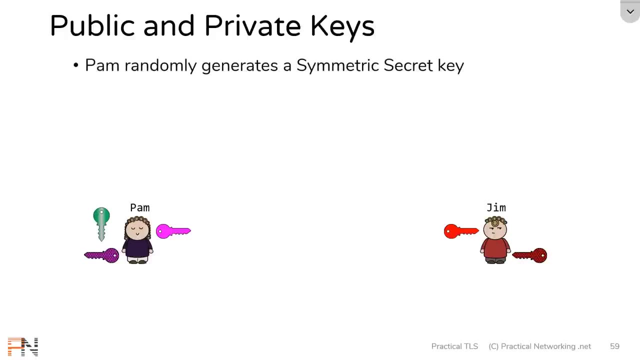 encryption for smaller, limited data sets. Well, why don't we use asymmetric encryption for smaller, limited data sets? an asymmetric key pair to share a symmetric key. that is what SSL and TLS actually do. let me show you how it works. Pam is going to randomly generate a 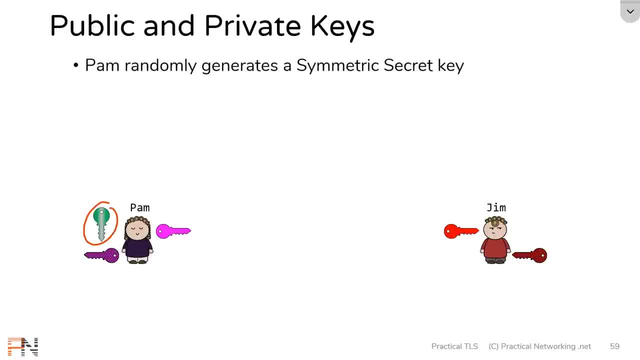 symmetric secret key. this key is just a string of ones and zeros and Pam will generate them randomly. Pam will then take Jim's public key and encrypt that symmetric key. the only key in the world that can decrypt this back to the original symmetric secret key is Jim's private key, which only Jim has, which. 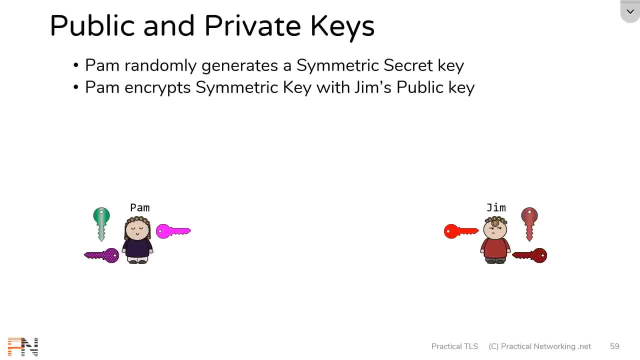 means Pam is safe to send that across the wire. Jim will then take his private key to decrypt the content of that message, to extract the original symmetric secret key. and now both parties have established a symmetric key that is identical in a secure way they can use that. 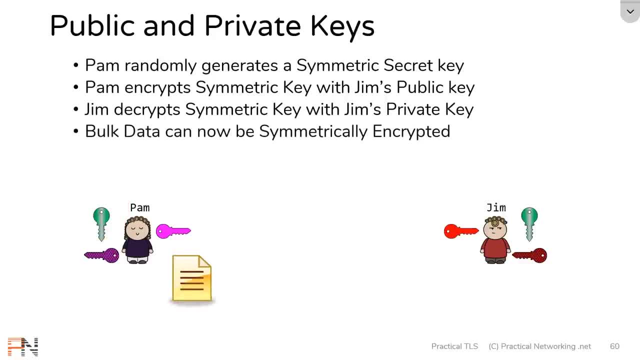 symmetric key to decrypt it, key to protect bulk data. Here Pam has a message for Jim. Pam will encrypt that message with her symmetric key. The only key in the world that can decrypt that message is the same symmetric key that was used to encrypt it. That message can. 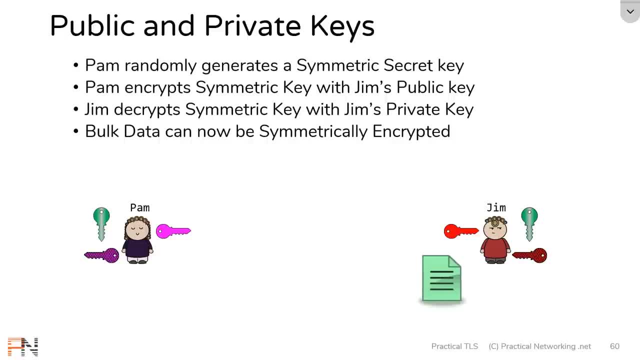 be sent across the wire, and then Jim can use his copy of the symmetric key to decrypt that message and extract the original content. This can be done in either direction for an arbitrary amount of data. Here Jim is sending something to Pam securely using that same symmetric key. Now that both parties have the 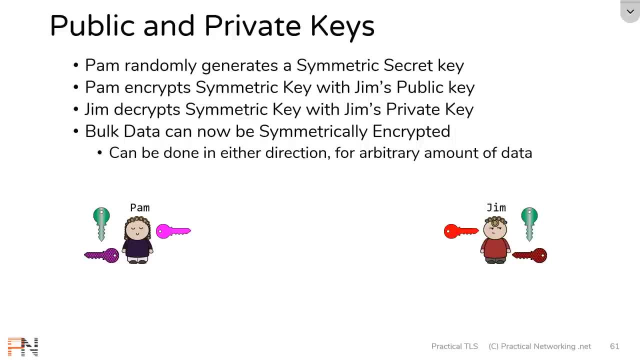 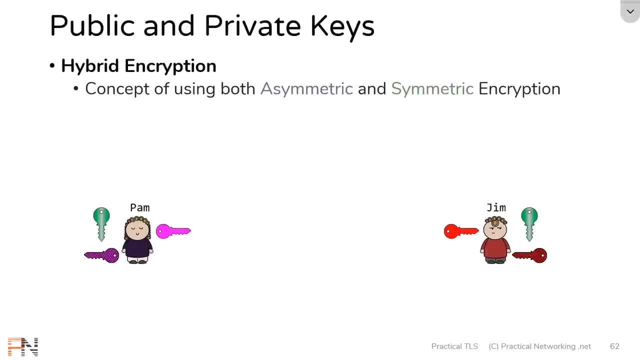 identical symmetric key on either side. they can continue to use that for however much data that they want to protect. This concept that we just discussed is referred to as hybrid encryption. Hybrid encryption is the idea of using both asymmetric encryption and symmetric encryption. Now you're using both of those at different points, so it's not like you're. 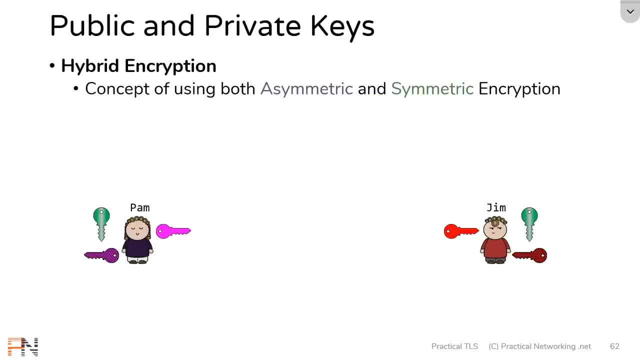 both symmetrically and asymmetrically encrypting the same content. You're using asymmetric encryption to facilitate a key exchange and then, with this key, you are then using symmetric encryption to protect bulk data. Do you remember those strengths and weaknesses of symmetric and asymmetric encryption we talked about? 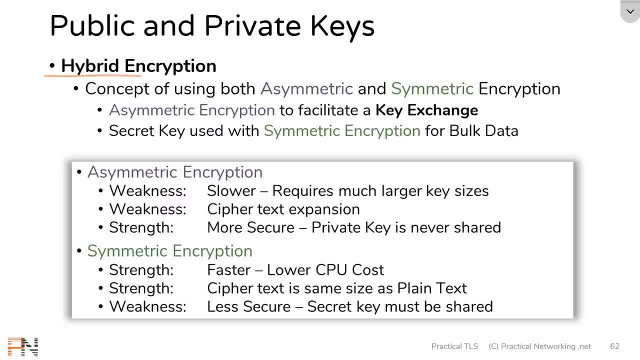 in the last lesson. Using hybrid encryption in this way gets you the best of both worlds. You get the strength of asymmetric encryption that you have used, the more secure way of sharing a key, and the efficiency of symmetric encryption to protect your bulk data transfer. This 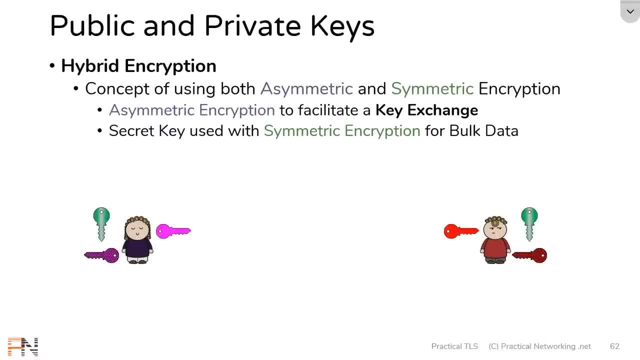 method is what every secure communication protocol uses. This is how SSL and TLS protect bulk data transfers. This is also how IPsec and SSH protect bulk data transfer. So that is the concept of hybrid encryption. But what about signatures? We talked about earlier how you can use signatures to attain integrity and 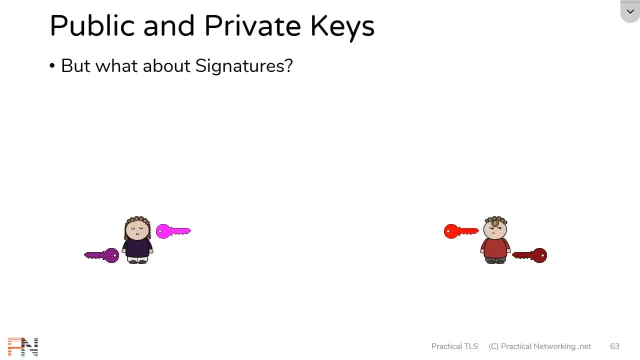 authentication on a message by encrypting something with your own private key. But again, asymmetric encryption has limitations. You can't simply encrypt an entire message with a private key. Instead, what we'd like to do is simply encrypt a smaller, fixed, representational sample of that message. 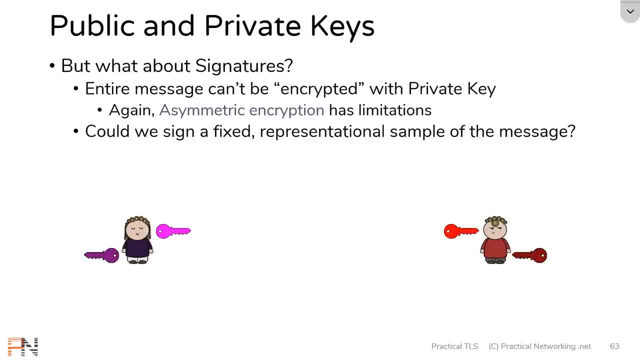 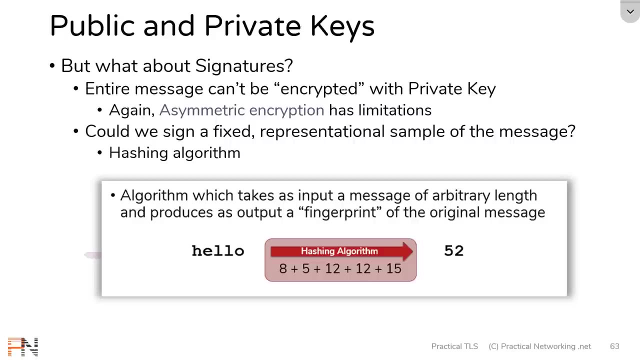 If only we had a way of converting messages to smaller representational sizes. Well, we do. We talked about hashing algorithms earlier on in this course. We define them as a thing that specifically exists to take a message of any size and produce a smaller fixed width fingerprint of the original message And signing is. 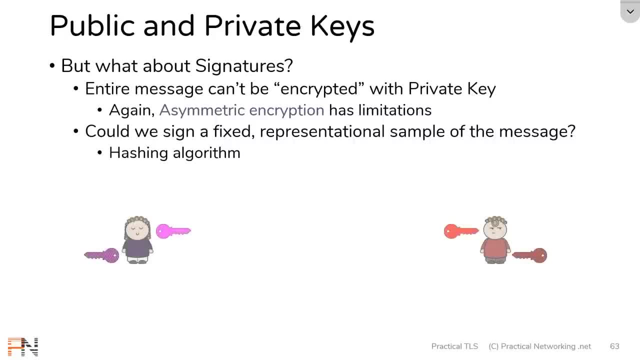 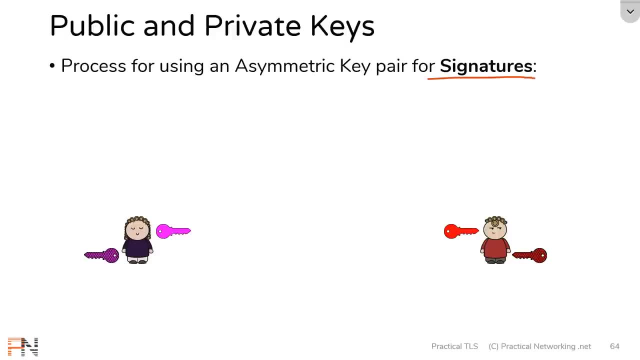 going to use hashing algorithms to simplify the process. Let me show you how that's going to work. Here is how asymmetric keys are used for generating signatures. Pam is going to generate a message. She has the permission to have personal houses. She is then going to run that. 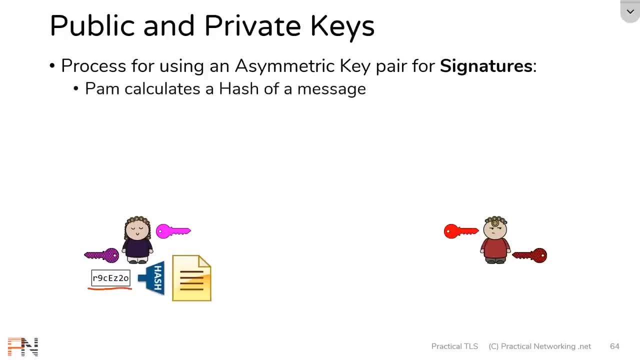 message through a hashing algorithm That's going to result in a particular digest. That digest is then going to be encrypted with Pam's private key. The result of that, which is the encrypted digest, is the signature. that is actually the signature of that message, That gets appended to the message and 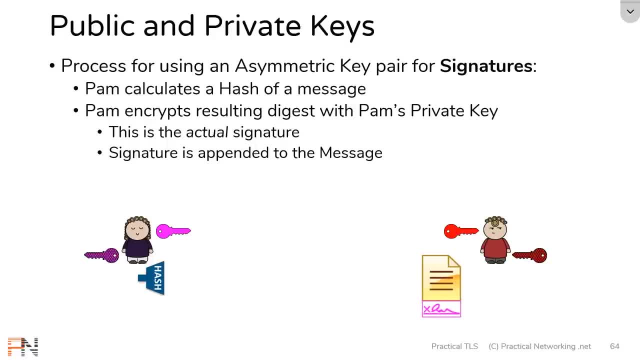 then both the message and the signature get sent across the wire And that signature was creator with Pam's private key. Now that signature was created with Pam's private key, which means he's already having a rather missingkey on that'Signature. This is really just. 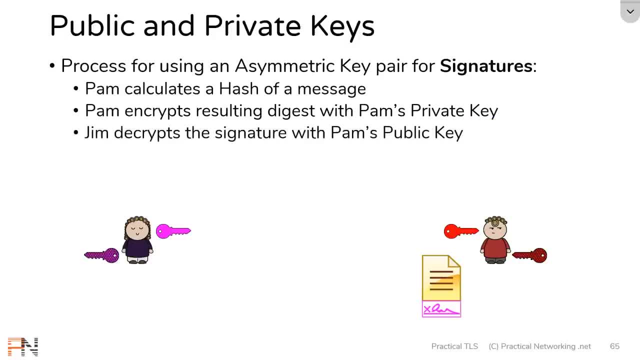 on the other side, Jim is going to use Pam's public key to verify the signature. What he's going to do is take the signature and decrypt it using Pam's public key. That's going to result in the digest that Pam created. Then Jim is going to independently calculate a hash of that message. 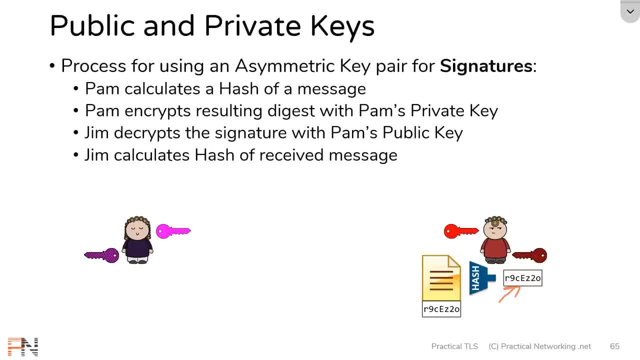 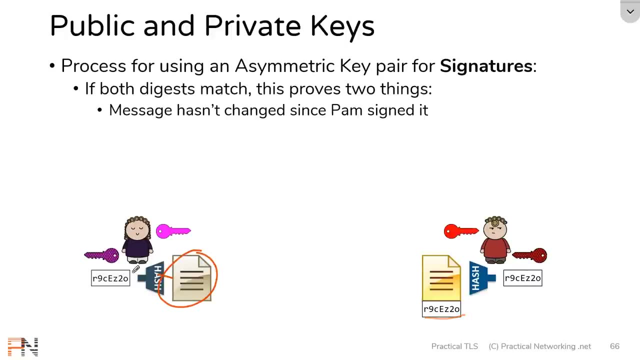 And if the digest that Jim got in his calculation matches the digest that Pam had sent, this proves two things. First, it proves that the message has not changed since Pam signed it. Remember, this digest was created by taking a hash of this message. So if anything changed, 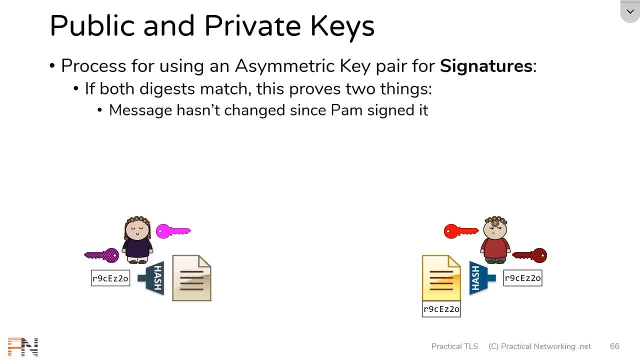 in this message, Jim would have gotten a different digest. This gives us the property of integrity. The other thing that signatures prove is that only Pam could have created the signatures. This signature was created as a return agent result of taking PAM's private key and encrypting this digest. Well, if Jim was able to decrypt, 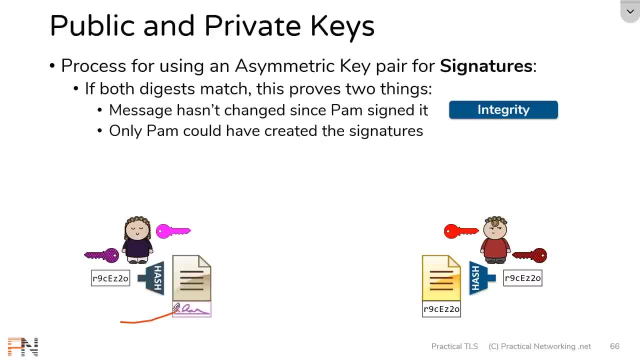 something with PAM's public key. this proves it was definitely PAM's private key that signed it, And the only person in the world that has PAM's private key is PAM. This gives us authentication. So using an asymmetric key pair to generate signatures in this way gives us both integrity. 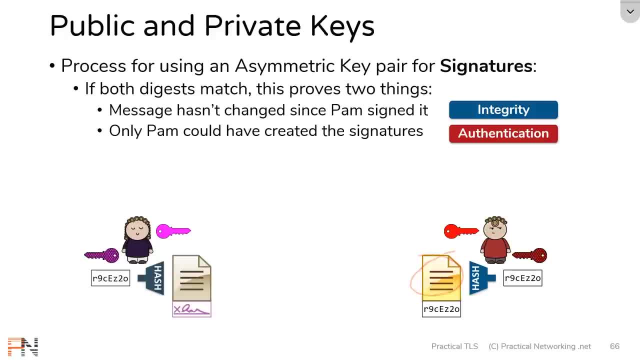 and authentication for the content that was signed. Now we've been discussing this from the perspective of a message sent across the wire, But keep in mind many different things can be signed. Sure, you can sign messages, but that's actually pretty rare. Often what you see signed,